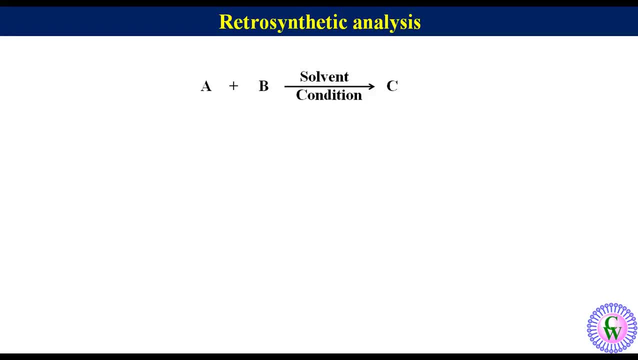 reaction condition to produce C, then you can easily predict the structure of C. For example, suppose someone asks you to predict the structure of product when acetophenone is allowed to react with sodium borohydride in ethanol at 0 degree centigrade to RT. Here we know that sodium 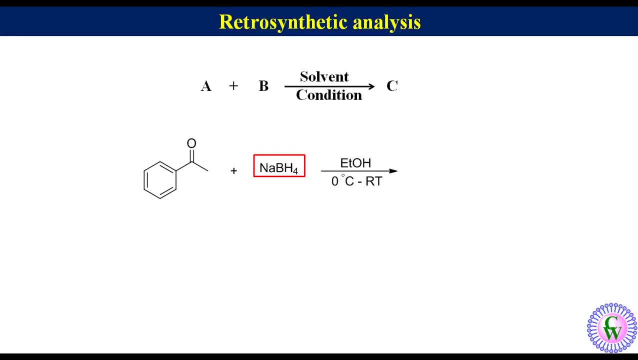 borohydride is a reducing agent that will reduce keto group to alcohol. So we reduce the keto group of acetophenone to alcohol to get the structure of the product, which is 1 phenyl ethanol. Similarly, if we are asked to predict the structure of product, 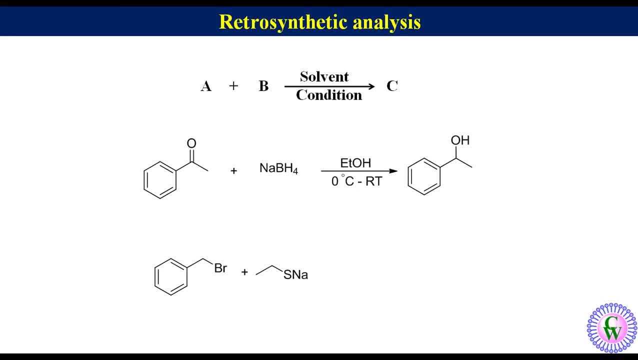 if benzyl bromide is allowed to react with sodium thioethoxide in DMF solvent at RT, then we know that sodium thioethoxide is a nucleophile, So it will attack on benzyl bromide via SN2 mechanism to produce benzyl ethyl thioether. The situation becomes bit difficult when you 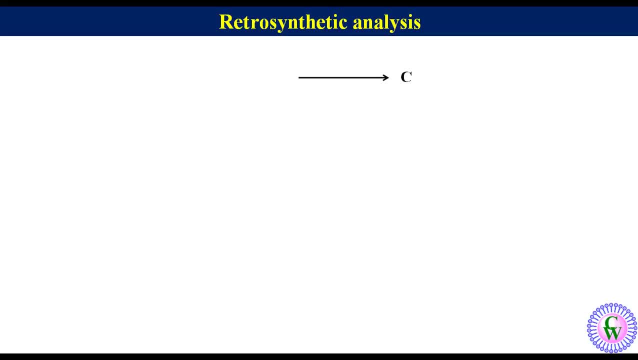 have to synthesize a product molecule which has a fixed and unchangeable structure. In that situation you have to work backward towards the starting material. This process is called retrosynthesis, and the art of planning the synthesis of a molecule is called retrosynthetic. 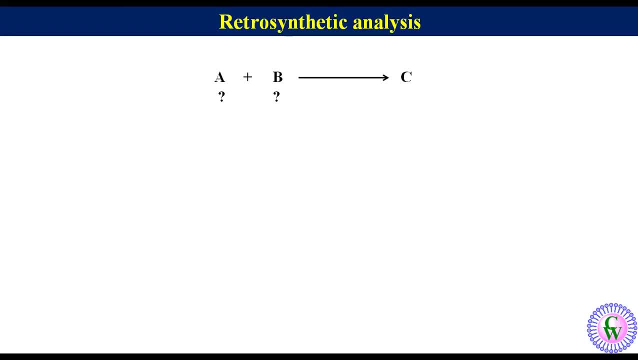 analysis. Synthesis of a target molecule may involve one or more than one step. Here we will first learn the retrosynthetic analysis of one step, and then we will learn the process, and after that for multiple step synthesis. Lets first learn different symbols and terminologies. 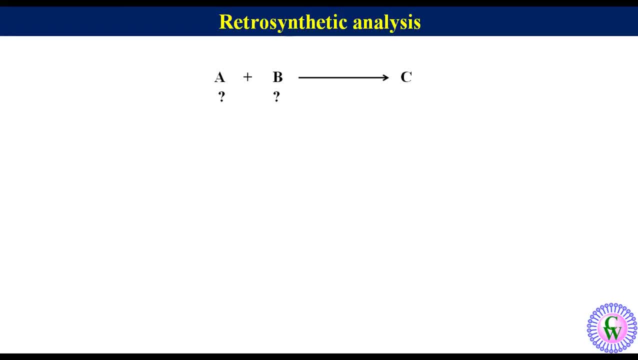 used in retrosynthetic analysis. Lets first talk about retrosynthetic arrow. This is an open ended arrow. The general meaning of this arrow is: can be made from. Lets have a hypothetical reaction in which A reacts with B to produce product C. 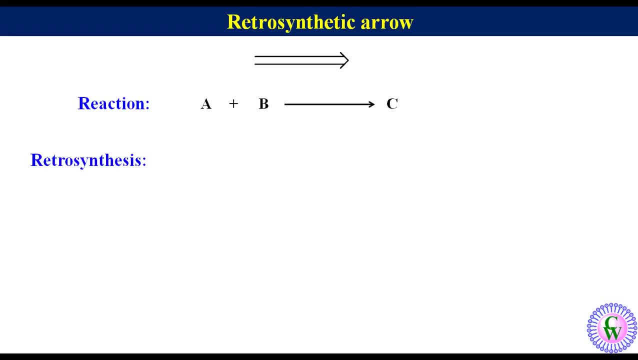 The retrosynthesis of this reaction can be represented as C retrosynthetic arrow. This means C can be made from A and B. Lets have a real example: Benzyl chloride, when allowed to react with methanol, produces methyl benzoate. It can be retrosynthetically represented. 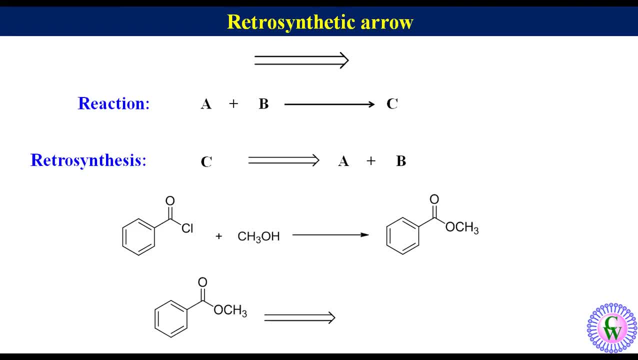 as methyl benzoate, then produced by Rich-Evening temperature Disconnection –. It is an analytical operation which breaks a bond and converts a molecule into possible starting materials. This is the reverse of a chemical reaction. It is represented by R university rate, E degree and V odd connector of A rate. You期 find. 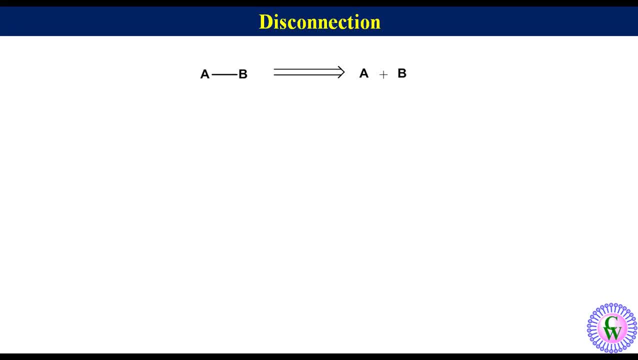 a retrosynthetic arrow and a curved line drawn through the bond being broken. for example, paracetamol, it's an amide. we can disconnect this amide bond like this to get the starting materials: four aminophenol and acetyl chloride or four aminophenol and acetic anhydride. 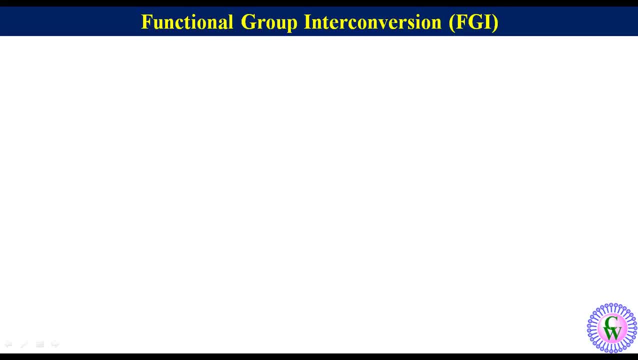 functional group interconversion. sometimes what happens that the disconnection of a bond doesn't lead to the logically starting material. in that situation, one functional group is replaced by another to make the disconnection possible. the operation of writing one functional group for another so that disconnection becomes possible is called functional group interconversion. 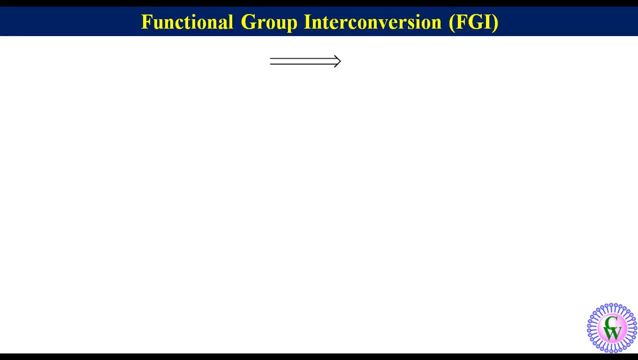 it is represented by a retrosynthetic arrow with fgi written over it. for example, replacing aromatic amine group with nitro, as amine can be obtained by the reduction of nitro. replacing aromatic carboxylic acid group with aromatic methyl carboxylic acid with nitrile primary amide with nitrile amine with imine primary amine with. 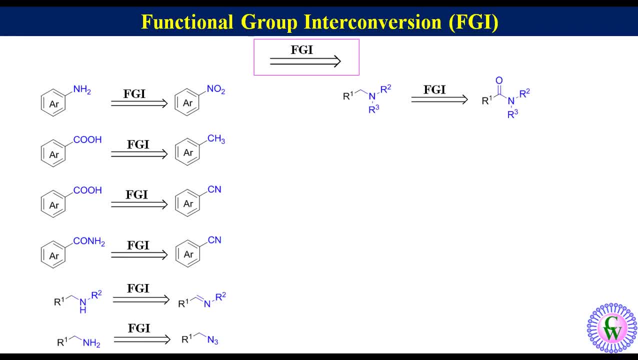 azide amine with amide amine with nitrile, carboxylic acid with alcohol, diol with alkene, keto with alcohol, etc. let's have an example where we can see the significance of functional group interconversion. suppose we have to do the retrosynthetic analysis of three bromoaniline 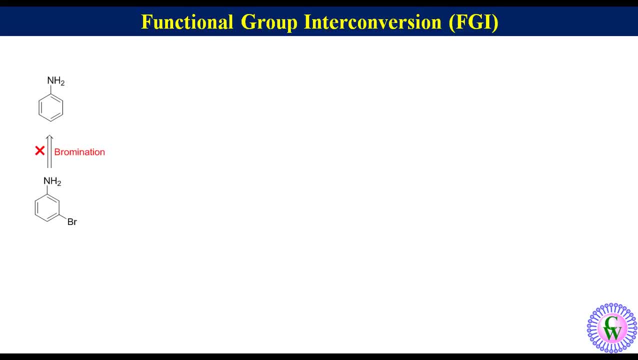 here. we cannot get it from the bromination of any leen because amino group in any leen is orthopara directing. so we can say that the disconnection of cbr bond is not possible in three bromoani lean. but if we do functional group inter conversion of amino to nitro group. 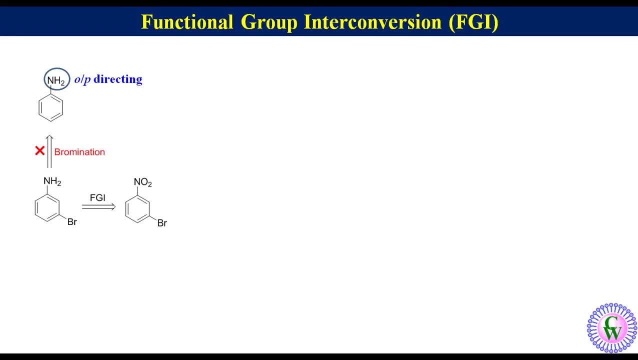 to get three bromo nitróbenzene. the disconnection of cbr bond is quite possible because we can get 3 bromcraft, newer group nitrobenzene by the bromination of nitrobenzene using Br2FeBr3.. Further we 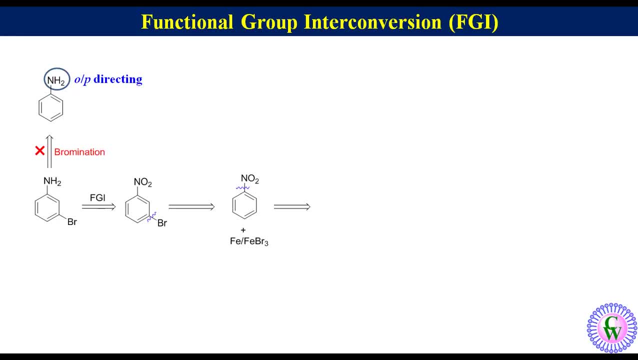 can disconnect this Cn bond because we can get nitrobenzene by the nitration of benzene with nitrating mixture. Thus we can start the synthesis of this compound from benzene. The first step is nitration to get nitrobenzene. 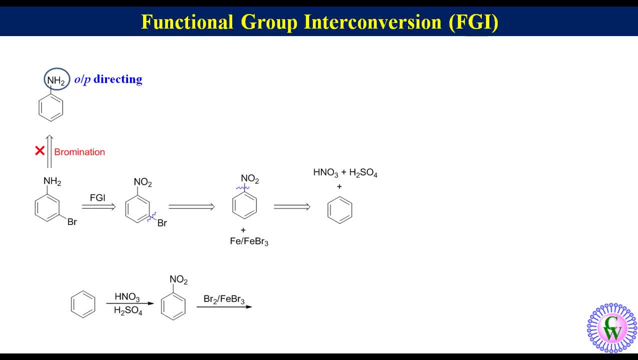 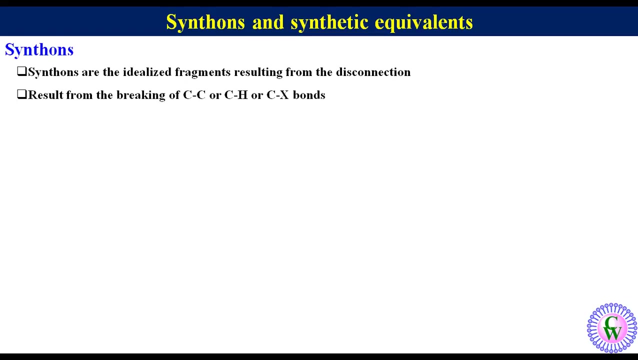 After that, bromination to get 3-bromo-nitrobenzene, and then reduction using iron and ammonium chloride to get target molecule Synthons and synthetic equivalents. Synthons are the idealized fragments resulting from the disconnection, That is, the fragments resulting from the breaking of Cc, Ch or 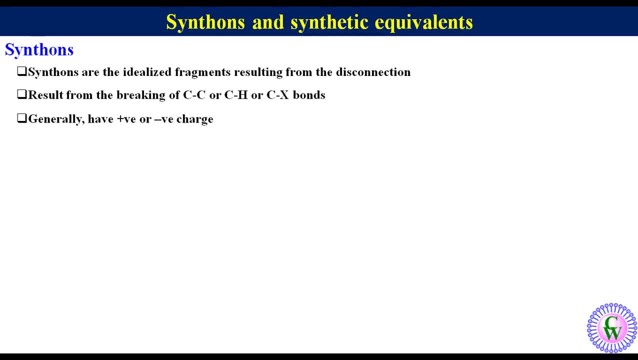 Cx bond. They generally bear positive or negative charge. These are not actual reagents. Synthetic equivalents, also called reagents. These are the actual compounds that are equivalent to synthons. Basically, they act as sources for the synthons. For example, if we have 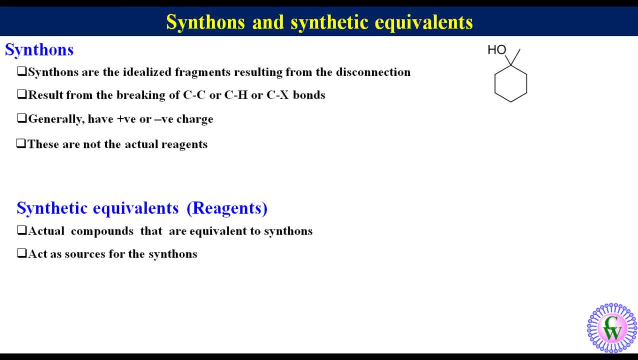 to do the retrosynthetic analysis of 1-methyl cyclohexanol. we can do this connection here to get hydroxycyclohexane-1-illium-catan and methyl carbonan. These two fragments will be called as synthons. The actual reagent for the carbocatan is cyclohexanone and 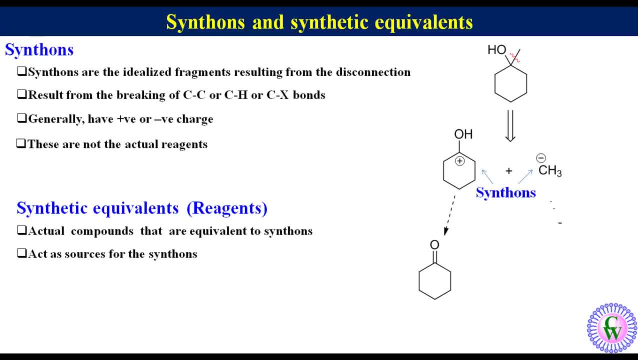 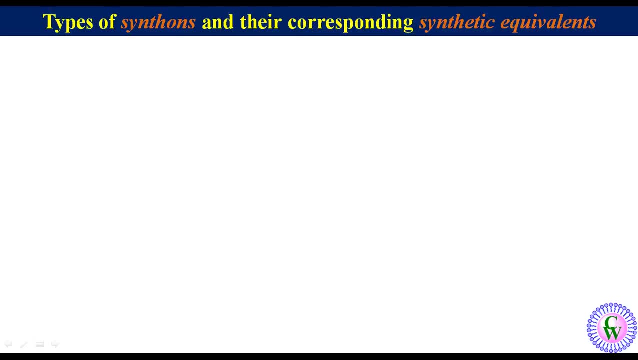 the actual reagent for methyl carbonan is methyl magnesium bromide. Thus cyclohexanone and methyl magnesium bromide will be synthetic equivalents. We have just seen that disconnection generally gives positively charged and negatively charged fragments which are electron acceptors or electron donors. 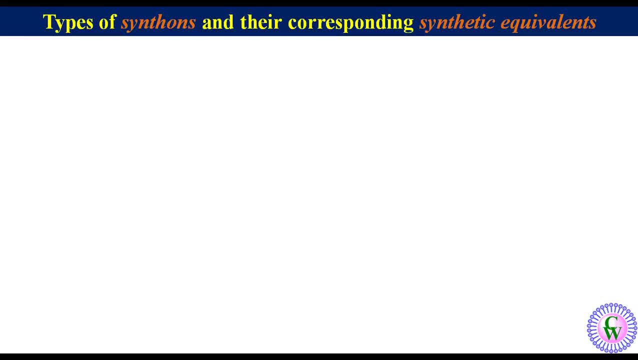 respectively. Based on that, we can classify synthons as acceptor synthons and donor synthons. Let's take one by one. First, acceptor synthons. These are positively charged fragments. They act as electrophiles. Let's have examples of some acceptor synthons and their corresponding 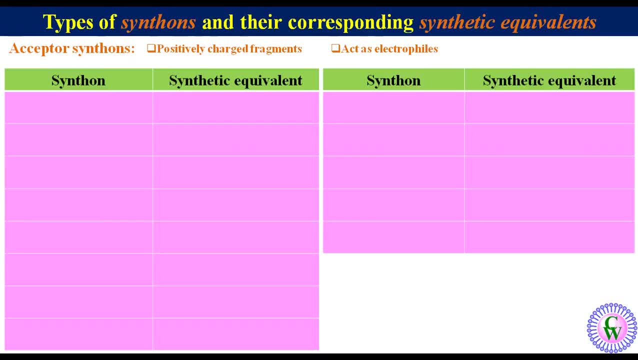 synthetic equivalents. Synthetic equivalents for alkyl cation or alkyl halides or mesylates or tosylates or triflates For aryl cations, aryl diazonium salts, fluoro or chloroarenes For oxomethulium ion. 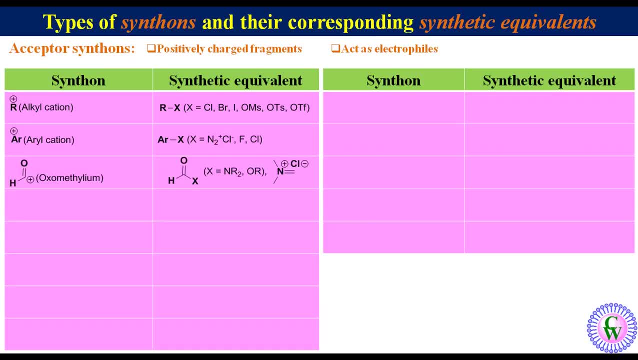 n-n-dia-alkyl-pharmamide alkyl format or willsmei salt For oxoalkylium ion. n-n-dia-alkylamide, ester, acyl chloride and anhydride. 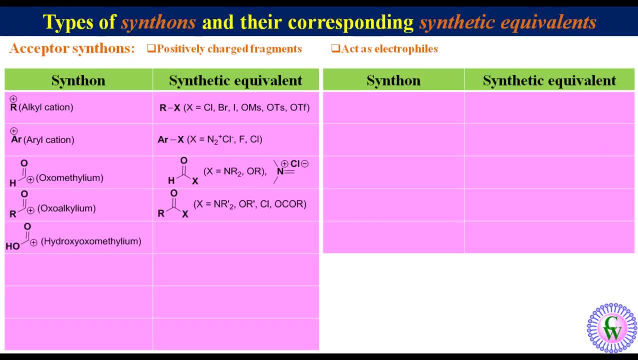 For hydroxy oxomethulium ion. carbon dioxide for hydroxy ion. formaldehyde for hydroxyalkylium ion. aldehyde for hydroxydialkylmethylium ion corresponding ketone for 2-hydroxyalkane 1-elium ion. epoxide for the beta. 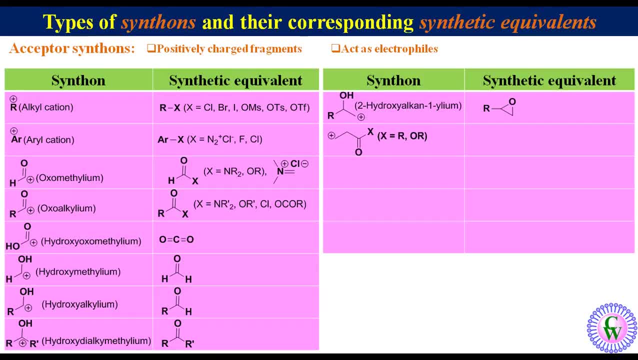 carbocation of ketone or ester alpha beta unsaturated ketone or ester for the beta carbocation of nitriles- alpha beta unsaturated nitrile. for alpha carbocation of ketone or ester alpha chloro or alpha bromoketone or ester for alpha. 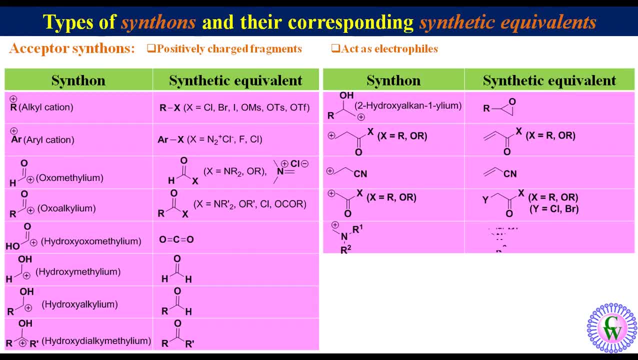 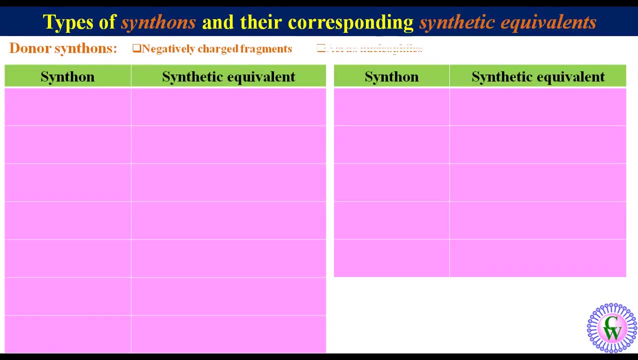 carbocation of secondary amine iminium ion that can be generated in situ by the reaction between formaldehyde and secondary amine Donor synthons. these are negatively charged fragments. they act as nucleophiles. Let's have some examples of donor synthons and their 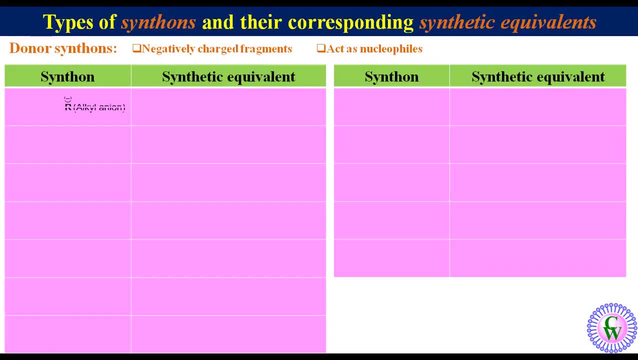 corresponding synthetic equivalents. Synthetic equivalents for alkyl anion are Grignard reagents, alkyl lithiums or Gilman reagents. All these three can be derived from alkyl halides. For the aryl anions: Grignard reagents, aryl. 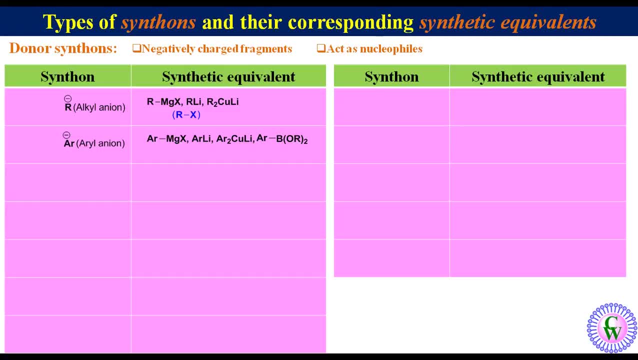 lethaims, Gilman reagents and aryl boronides. anion can be obtained from aryl halide too. All these four can be obtained from aryl halides. For alkynyl anion, the synth improvements are alkyl, alkynyl halide and alkynyl boronides. For acetyl tanks, Inira��요 lawyer select'the asymptoticringe or wolf RT. or the second nutrient, collocate alkyl boronaideze at ethyl halidedewel, ecetylene and الإnion in the anion as cl son driving anion For alkynyl anons. the synthetic equivalents are shelf marine ions. Columbiano す, VanderSi, Hardy O, Nina et alA overtake alkynyl halide and Alkacyl boronidae. 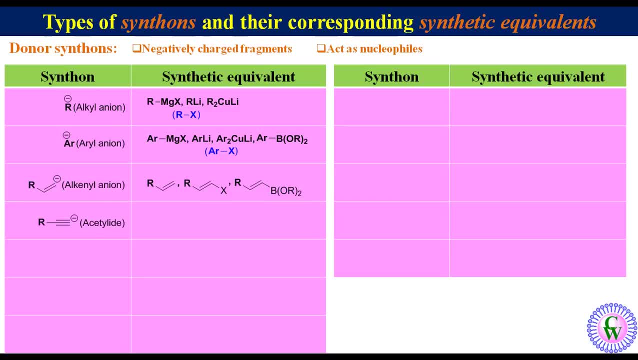 For Acetylite, Lithium, Sodium or Copper. Acetylites that can be generated from Terminal Alkynes. For Cyanide, Sodium or Potassium Cyanide. For Enolate Ketone or Beta Ketoester. For Sinomethyl Anion Acetonitrile or Sinomethyl Ester. 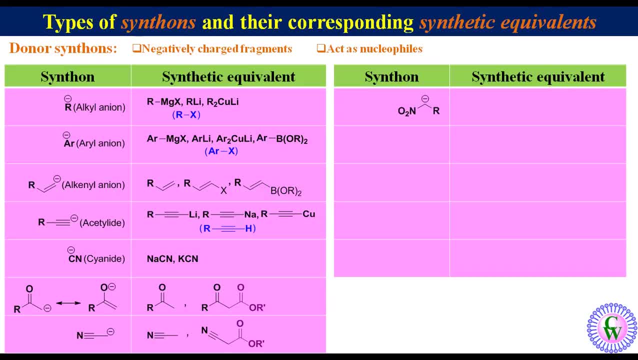 For Nitroalkyl Alpha Anion. Nitroalkane For Acyl Carbonion 1,3-Dithion or Nitroalkane For Wittig Elite Alkyl. Phosphonium Salt For Sulphonium Elite- Corresponding Sulphonium Salt. 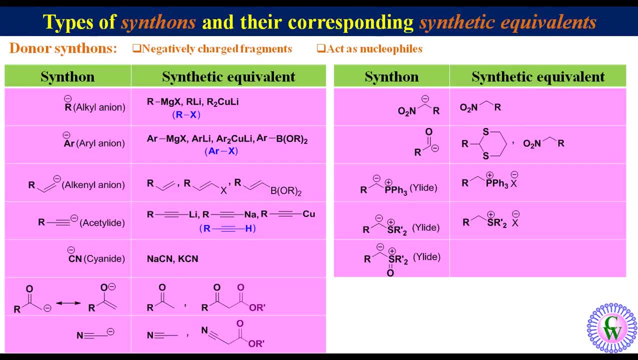 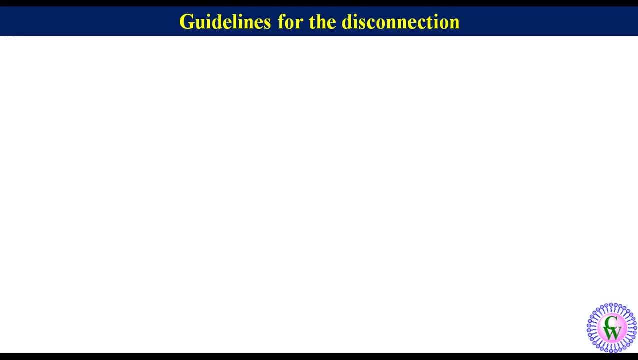 For Sulphoxonium Elite, Corresponding Sulphoxonium Salt. Guidelines for the Disconnection. The most difficult process of a Retrosynthetic Analysis is to find the bond to be disconnected. Here we will discuss some guidelines to help you out. 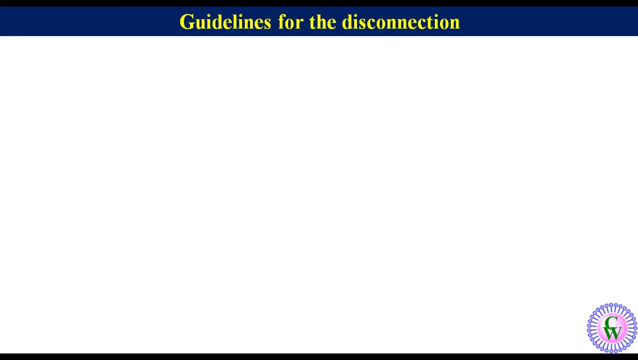